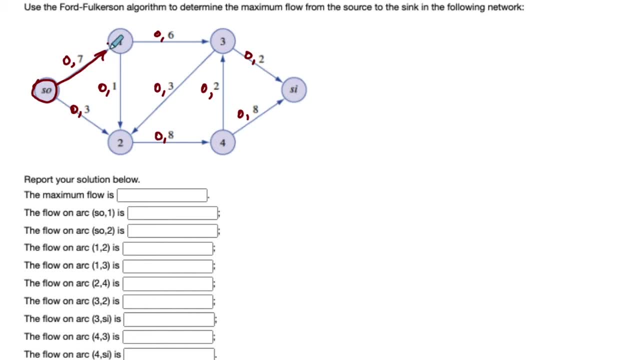 So therefore I can label node one by pushing the flow from source. All right, so once we labeled one, we are trying to label a next node which will take us a step closer to the system. So we can push some flow from one to three. all right, because again here we have zero flow on. 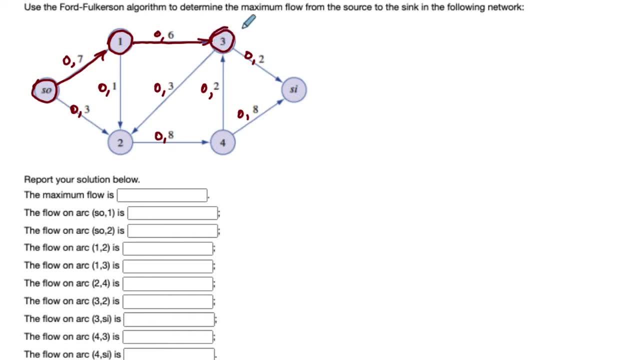 this arc right now and the capacity is six. so I could push up to six units, from one to three, Okay, and this way I label node three and then from three I could label the sink, and our goal is actually to label the sink and to send some flow from source to sink through this path that we 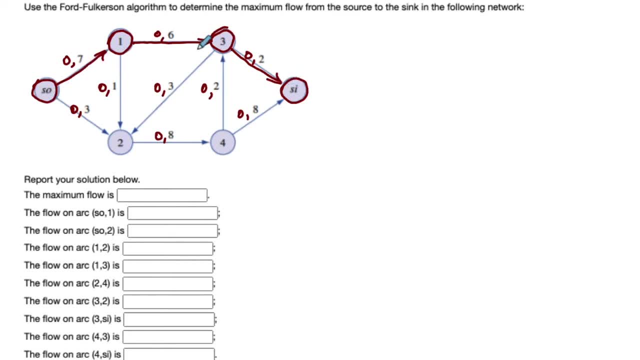 have already defined in our labeling procedure. So this is what we call the augmenting path, and we can augment the current flow by adding some more flow through this path. right Now, once you found the augmenting path, we need to determine the amount of the augmenting flow. 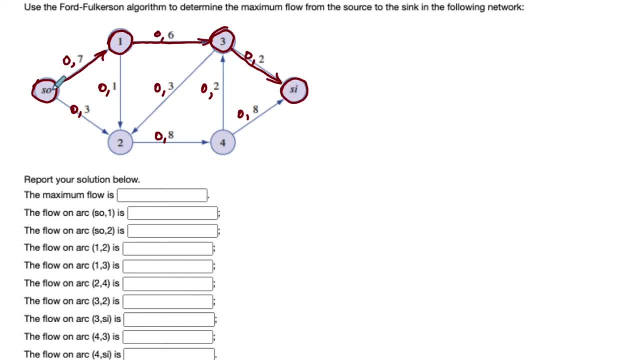 that we can send through this path and that flow is determined by the smallest remaining capacity among all the arcs in the path. right? So the smallest capacity would be for the arc three to sink. we only can send two units of flow here, right? so therefore we are. 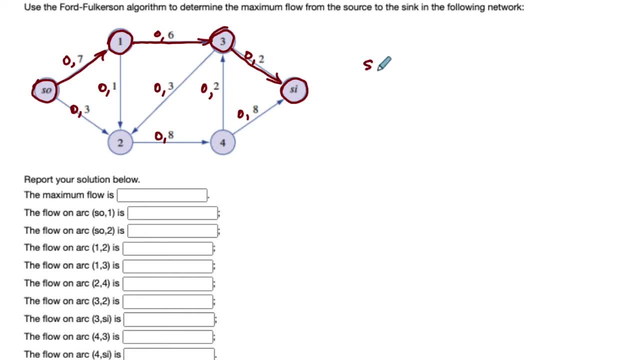 going to send two units of flow along the path from source to one to three to sink. so we send two units. All right, and I'm updating the solution accordingly. So I'm going to erase this path. Now, all this labeling, the trace of labeling that we have done, right? so I'm just going to update the flows now. 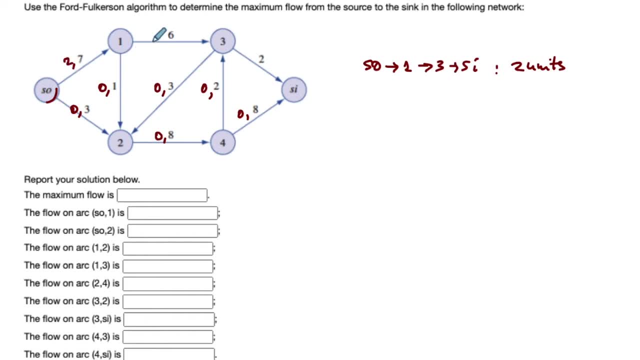 because now we completed the first iteration so we sent two units of flow along this path here. All right, so this is our updated solution. So next we start the labeling for the second iteration. so we label the source and from the source we are trying to find another. 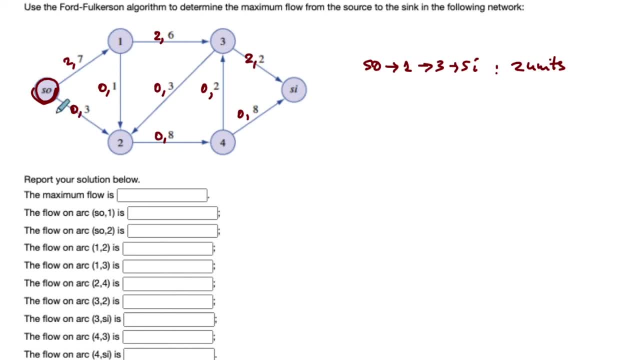 path to sync through which we can send some additional flow, and then there are a bunch of possibilities here. let's just pick some path that we can find so we could go from source to two, then from two to four- right, so then from four to sync. so this way we are going to label the sync. 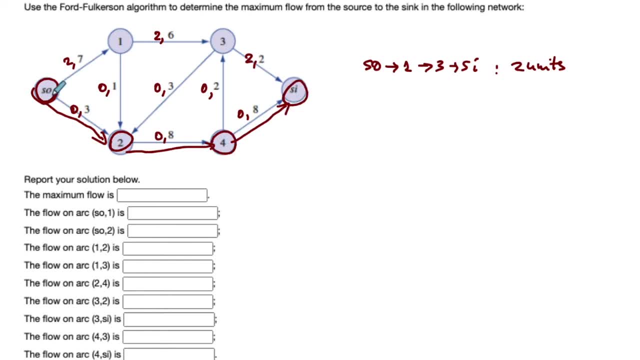 and then we need to determine again the augmenting flow, which will be again the smallest available capacity among all the arcs in this path here. and we can see that the bottleneck arc will be from source to two of the capacity three. so we are going to send 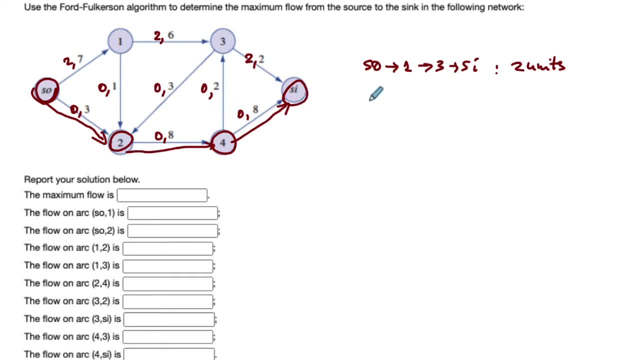 three units of flow through this path. so you'll go from source to node two to four to sync, and we are going to send the three units of flow through this path, all right, so let me remove again the labeling here and we'll update the flows. now. the flow on this arc is three. on this arc, it's three and on this arc it's three, all right. 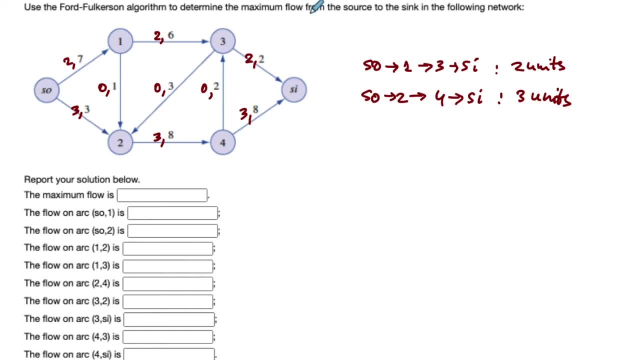 so now so far we are able to send five units of flow from source to sync right. so next we are starting the third iteration. so this was the first iteration, the second iteration. in the third iteration, again we start by labeling the source node and we can see that the only place 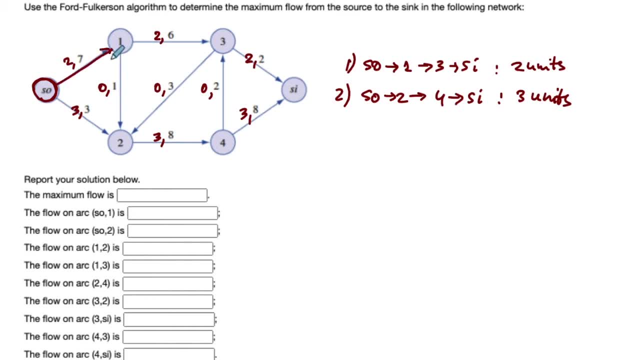 we can push now from source would be to node one, because here we already saturated this arc. there is no more remaining capacity. then from node one, there are possibilities. i could could either go this way or this way. so let's go again through arc one three as we did in the first. 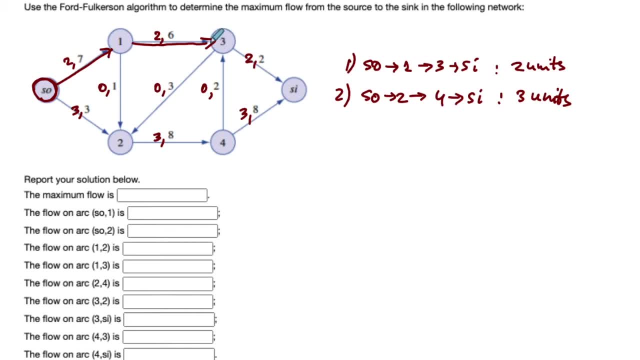 step, so we can send up to four units this way, right, and then from three- now i cannot go to sync because again, this arc is saturated, but i can go from three to node two, all right. so, and so far i labeled all these nodes and i can continue by labeling node 4 from node 2, because, again, i can. 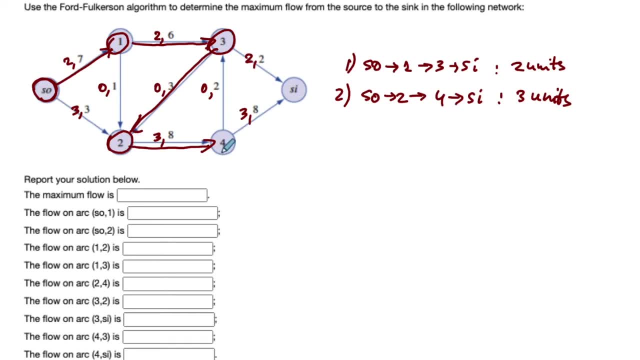 push some flow from 2 to 4 right, so we can label 4 and then from 4 we can label the sync. now in this path we are looking at the available capacities for the arcs and we see that we can push up to five units from source. 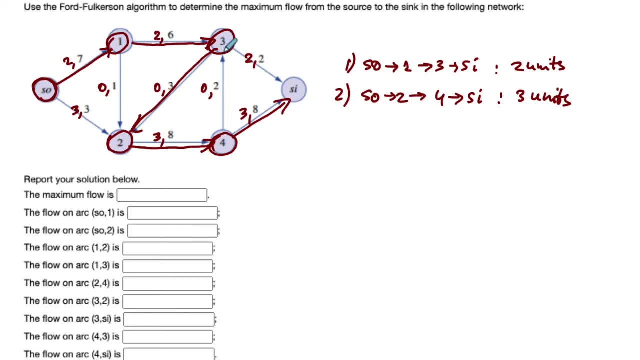 source to one, then four units from one to three, then three units from three to two, five units from two to four right and five units from four to sync. so we can see that the bottleneck Arc would be from three to two and we can send only up to three units through that Arc right. so this will. 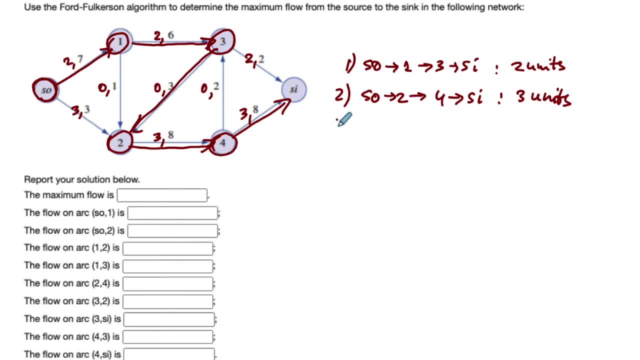 define our flow through this additional path here. so your go from source to node one, then to three, to two, to four and to sync, and we'll send three units of flow this way. okay, so I'm going to update the quantities now so we add three units of flow here, so from two 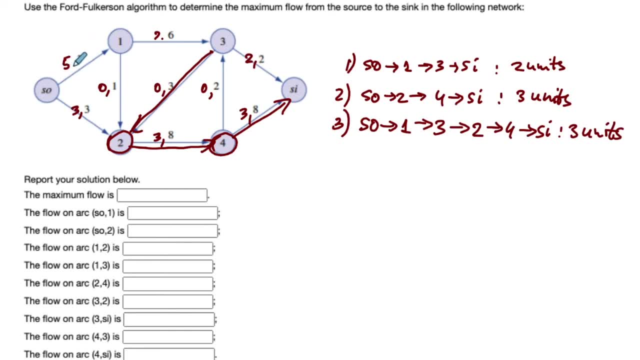 it goes to five. so here we are going, also from two to five. now, for this Arc is going to be three units. we go from zero to three. right then here the flow will increase from three to six and finally, along this Arc, we add three units of flow. so it's going. 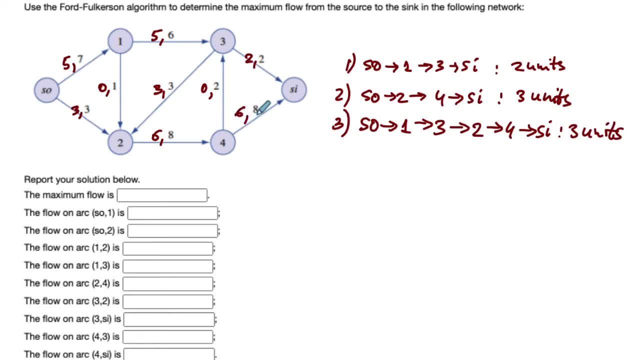 to go up from three to six. so we have this new solution now and we are ready for step four. so at step four we are labeling the source and we can label again node one from source, right. so because we still have two units of capacity that we can use for an additional flow. now from here I could go to three. 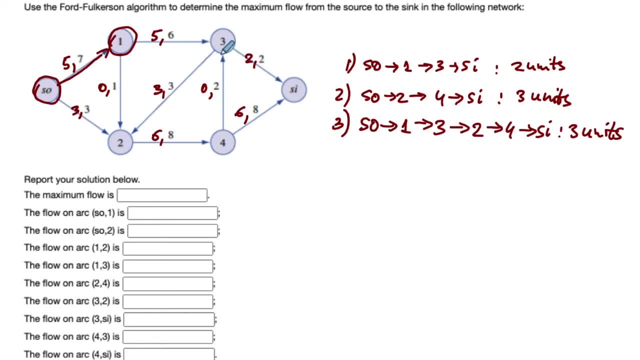 from three. there is nowhere to go. both of the outgoing arc are saturated, right? so let me label node two from one, all right, because we have one unit of capacity. going this way, then we can label four from two, because we have two units of capacity available, and sync from four, right? 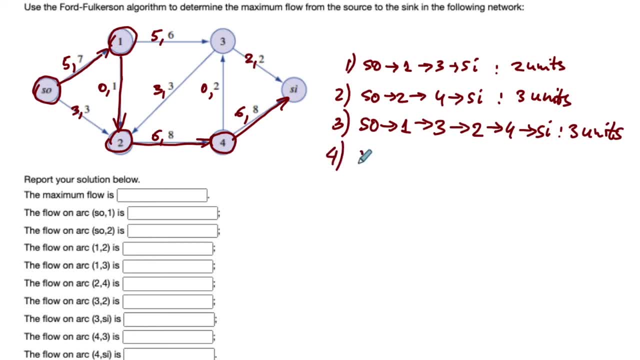 so our fourth augmenting path is gonna be source to one to two, to four, to sync, and we send just one unit because clearly the bottleneck arc will be one, two. there is only one unit of capacity available there, all right, and we can update now the flows on arcs for this arc, the 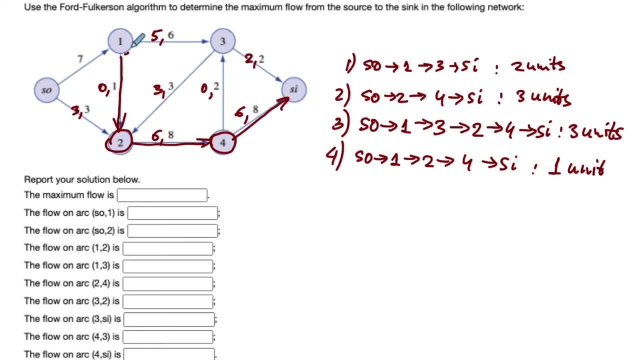 flow will increase from five to six. right. then for arc one, two, the flow is gonna be one now and we saturate this arc. then for arc two, four, we go from six to seven and from four to sync again, the flow increases from six to seven. all right. 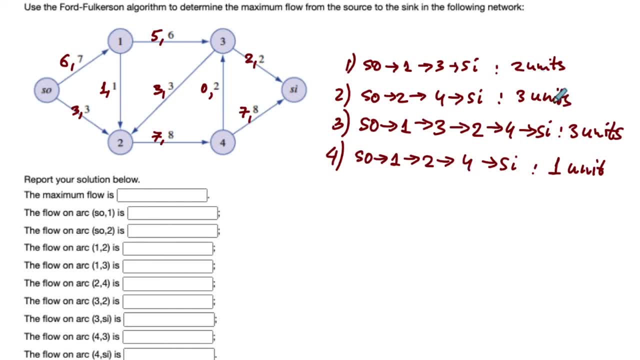 so now our current solution has nine units of flow sent from source to sync, right, so let's see if we can send more. we start the fifth iteration by labeling the source. from source, we can still label node one, all right. then from one we can label node three, only right, so there is no other node that. 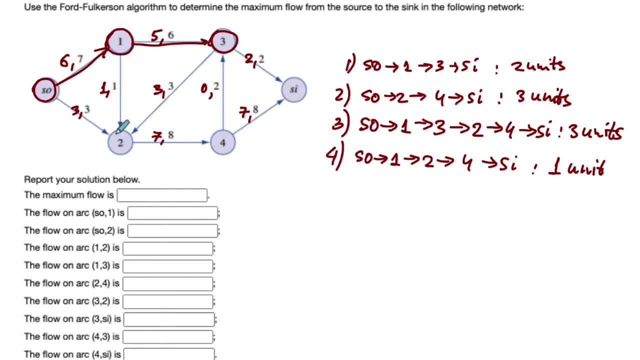 we can label going from one, okay so, but then from three, it looks like we are stuck. now there is no more capacity for us to move the flow right. so therefore, we conclude that this solution is optimal. and now, if you look at the cut between the nodes that we were able to label and the nodes that we 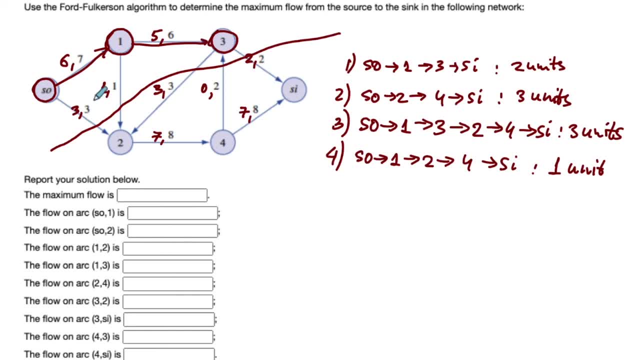 are not able to label, so the cut will be separated from the nodes that we were able to label. so we can see that we are now separating these three nodes from these three nodes, right, and if you look at the capacities of the arcs going from labeled nodes to unlabeled nodes, we can see that that capacity adds up to nine. so it's. 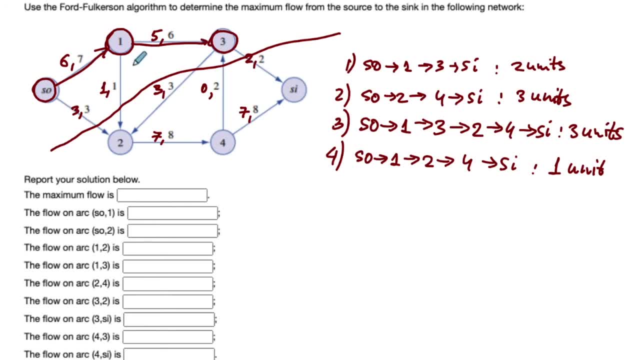 gonna be three plus one plus three plus two, right, so the total is nine and the value of the cut here is nine and the value of the flow that we have here. so therefore, clearly the solution is optimal. right. so we can report the solution now by looking at the flows that we have for every arc. so the 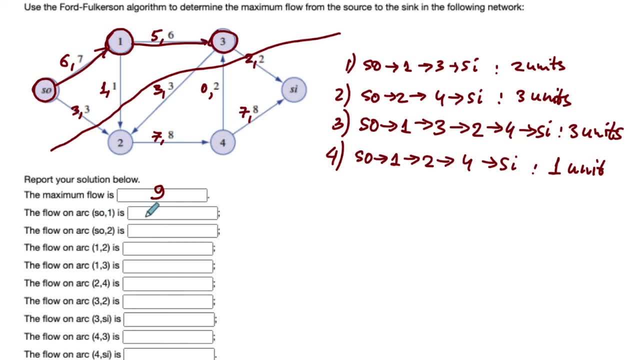 maximum flow is nine and the flow on the arc from source to one is six, then from source to two, it's three. from one to two is one to three, the flow is five. the flow on the arc two, four is seven, then on the arc three, two is three. 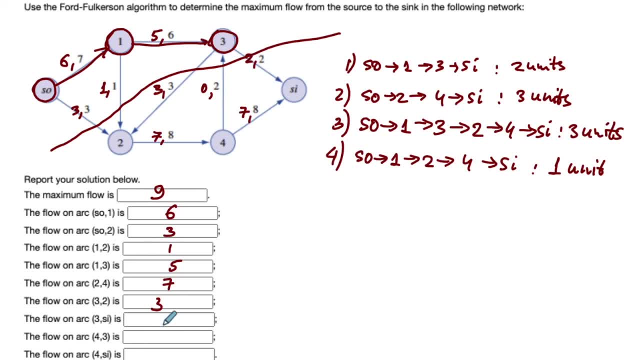 on three, sync is two. then on the arc four, three, the flow is zero. and finally, on the arc from four to sync, we have the flow of seven and we are done all right. so in this solution we only use the forward arcs in the labeling process. but now let's solve the same example by using some other augmenting paths where we encounter. 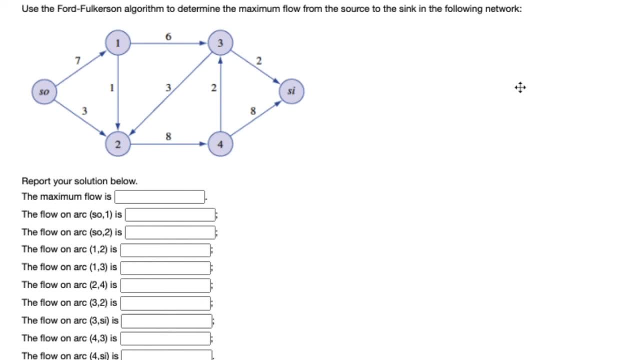 the backward arcs as well, just to illustrate the concept, all right. so in this case let's look at some other augmenting paths. so we saw that in our solution the flow along this arc here from four to three was zero. right, so now let's pick some augmenting path. 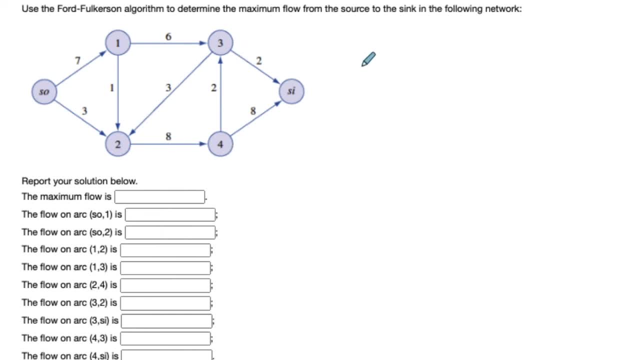 where we will push more than zero units along this arc so that this will result in a backward arc later on when we build other augmenting paths. all right, so let me take, let's say, the path on the first iteration, from source to two, to four, to three, to sync. 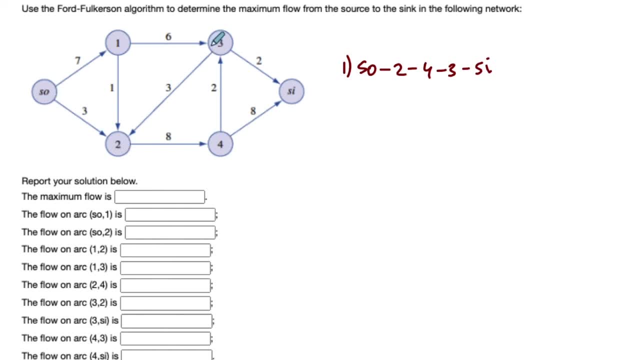 so we are going from source to two, to four, to three, to sync. let's see how many units we can push this way. only two units, right. so let me put the new flows here. so we send two units along this path, right next at the second iteration we could go, let's say, from source to node two- again right. 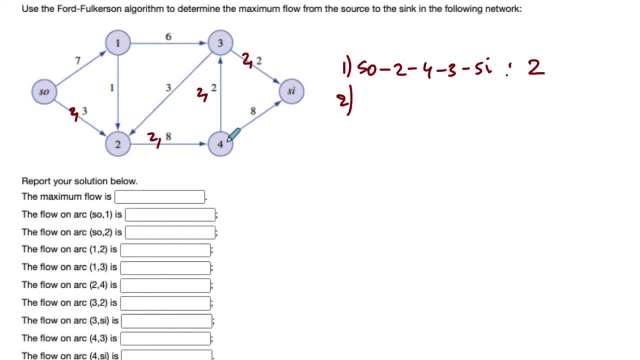 so from source to two, then to four and to sync, and we can see that there is only one unit of capacity remaining going from source to two. so this will be the bottleneck. we are going to add one more unit of flow here, so this will become three. so now we have one unit. 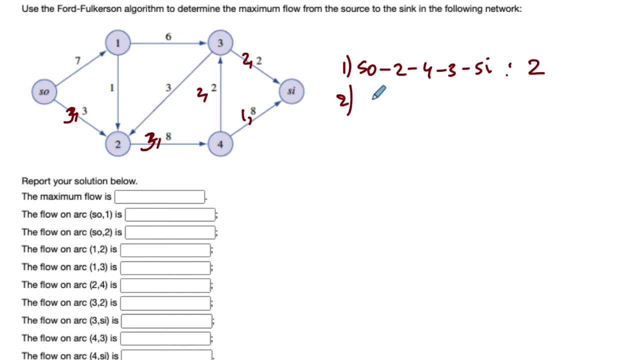 for this arc. so we added the flow along the path from source to two to four, to sin, we added one unit. all right, so this is our current solution. so next, when we are trying to label, the only way i can go from source now is to node one so i can label one from source, then from there. 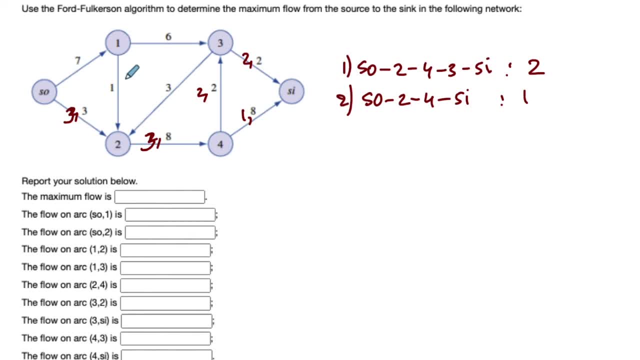 i could go to, let's say, two, then four and sync, right, so i could go from source to one to two, to four to sync, and let's see how many units i can push this way. so the bottleneck arc would be one, two, right, so we can only push one unit of flow here. so now the flow along this arc is one one. 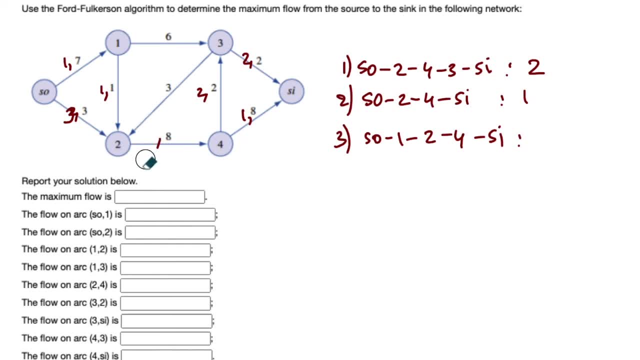 this will update to four next, and then the flow on the arc from four to sync will be two. now, so this was one unit of flow, all right. so next, what do we do? we label node one, again going from source. so the path that we can find is source to one to three. then from three we can go to two to four to sync. right, so this? 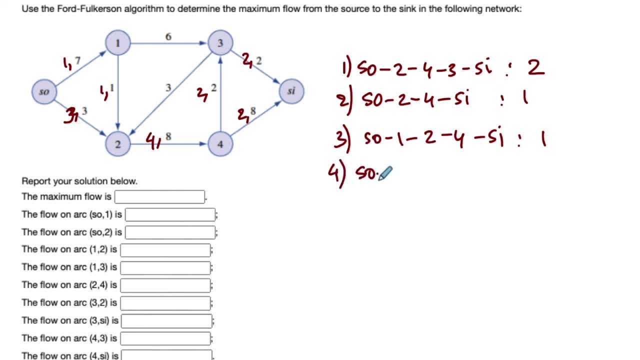 will be our fourth augmenting path, so it's gonna be from source to one to three, to two, to four. to sync, let's see how many units we can send this way. so up to six here, up to six here, up to three. so three is the bottleneck. 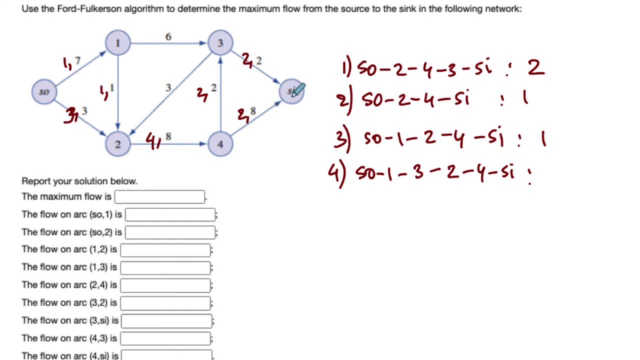 so far, then up to four units here, up to six units here. so three is our bottleneck. so we are going to add three units of flow this way, so this will update to four. then we have three units here, three units here, then we add three units here to become seven. 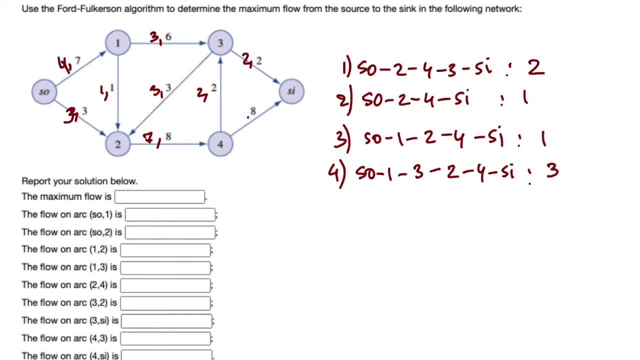 and three more. from four to six. we have five here. all right, so this is our updated solution, and now we are ready for the fifth iteration. so from source, we label one. now, the only way i can go from one would be to node three. all right, so you're avoiding backwards arcs as much as we could. so now i label three from three. 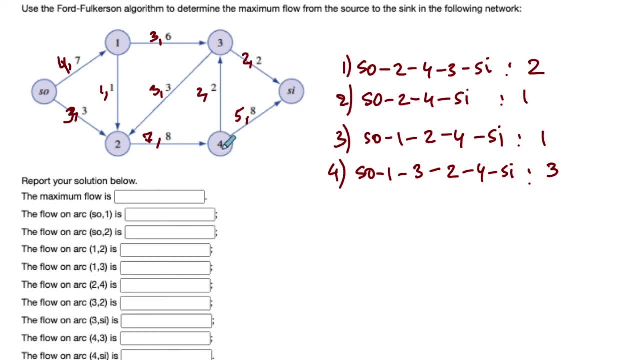 i don't have any forward arcs, but now i have a backward arc right, so i could push some flow back through this arc here. so right now i have two units of flow here. i could push these two units back and then from four i could push them to the sink right. so now we can go. 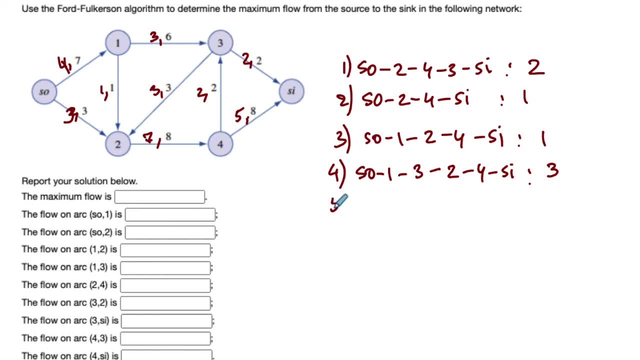 along this path, including the backward arc. so our fifth augmenting path will be from source to one to three to four, through the backward arc, right here, right, and then to sync. okay. so, and in this case, when we try to determine the bottleneck for backward arcs, we can push up to the amount of how much flow we have on that arc right now. 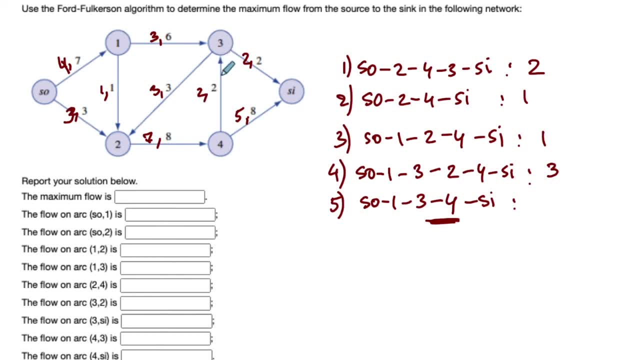 so we have two units of flow. so for this arc we cannot push back more than two units. right, so from this arc we can push up to three, up to three here, up to two here and up to three here. so this backward dark happens to be the bottleneck, right, so you can push up to two units through.